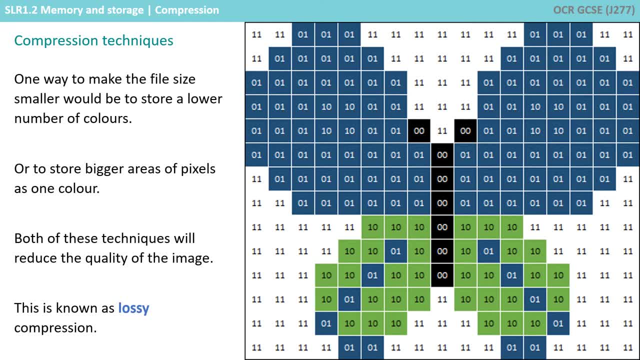 and therefore this is known as lossy compression. Algorithms such as JPEG and GIF, although very different, work a little like the two ways described With photographs and especially video. a lot of the images that are stored in a file size are stored in a lower number of colours. 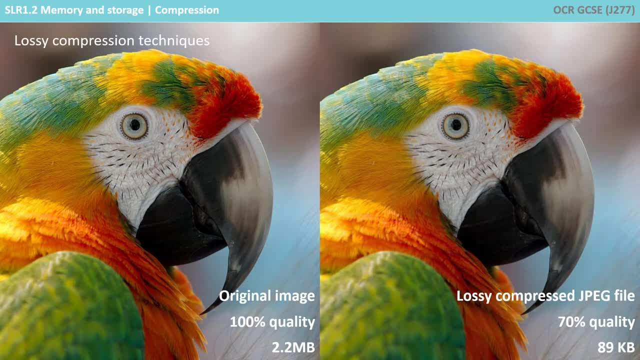 A little loss of quality might not be too noticeable and therefore it is considered an acceptable compromise of quality versus file size and download time. Here we can see two images, and it would be hard to tell that one is an original file and the other is compressed, but it has a significantly lower file size. 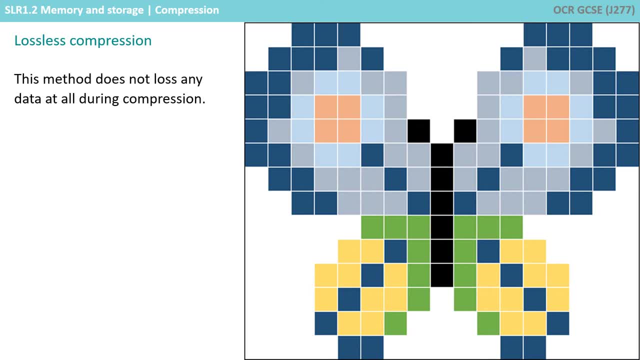 Another approach is not to lose any data at all. This is known as loss less compression, and it uses completely different algorithms. For example, in our original image of a butterfly, we can see that there are large areas of white pixels. Instead of storing every pixel with the same binary pattern, we could encode our data differently. 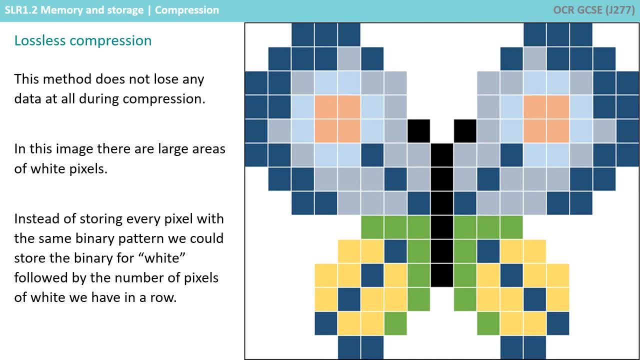 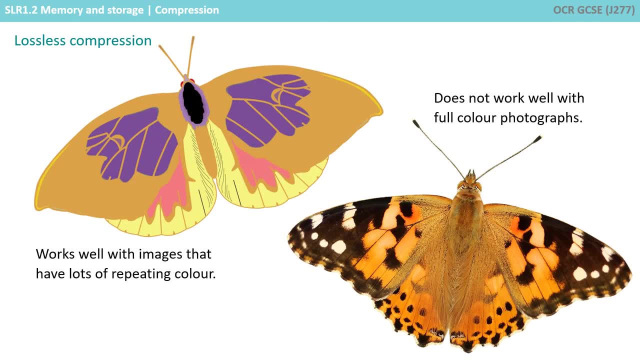 Perhaps by storing the binary for the colour white and then the number of white pixels in a row before the colour changes. Encoding data in this way would reduce the file size, but would only be effective on images with large areas of continuous similar colours. 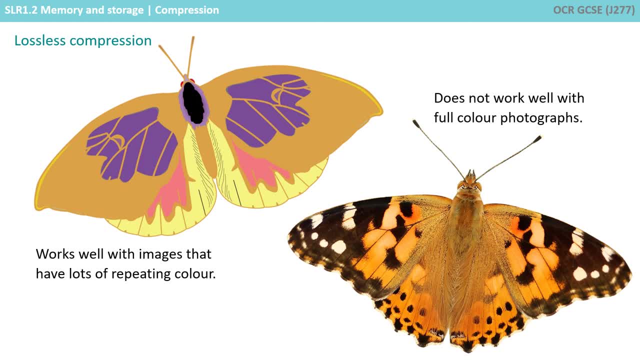 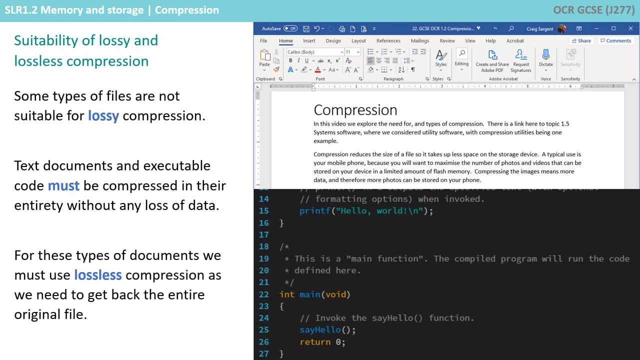 That makes it suitable for cartoons and clip arts, but ineffective with full colour photographs where there are few blocks of repeating colours. It's important to realise that the type of data will also determine what types of compression can be used, For example with executable program files. we cannot afford to. 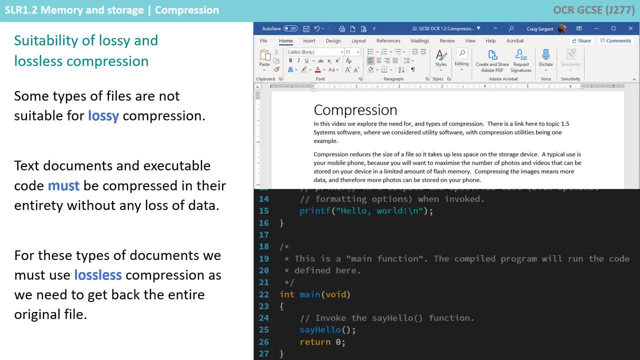 lose a single command in the program and therefore only lossless compression will work. This is also true of documents. It is really only with pictures, sound and video where lossy compression is applicable, but it does usually give us the highest return. Compression reduces the number of bits in a file. It makes the storage capacity of the file lower.